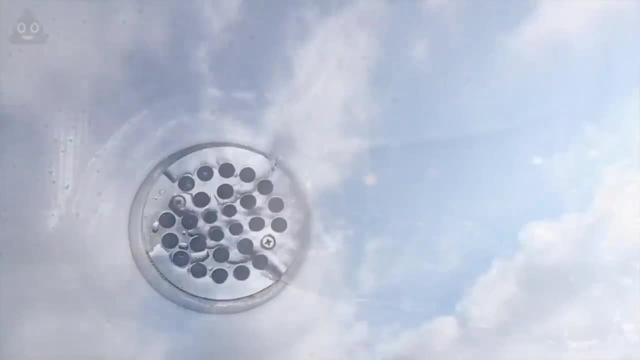 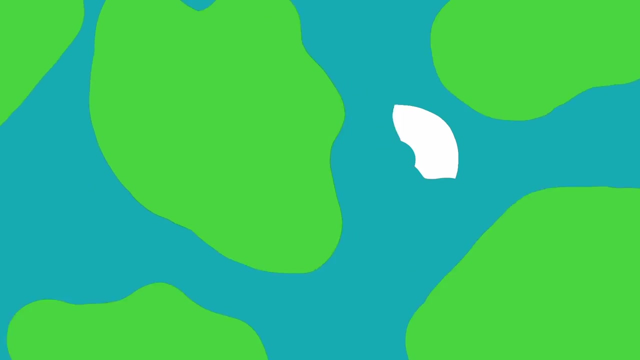 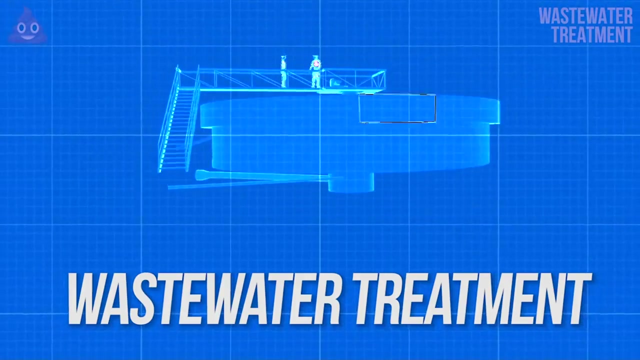 all dogs go to heaven. all drains in a city lead to a wastewater treatment plant, where the wastewater gets turned back into water that we can drink. Now you may be thinking you'd rather just let bygones be bygones and not think about that nasty part of real life, But here's the. 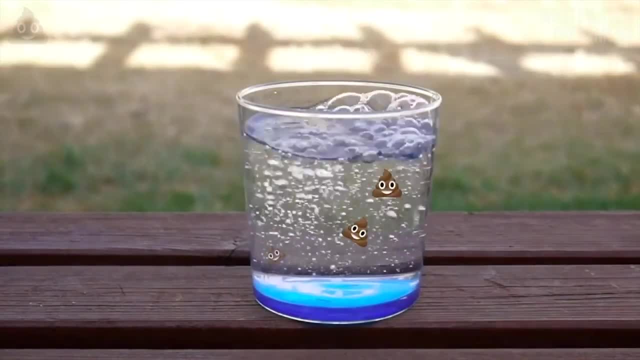 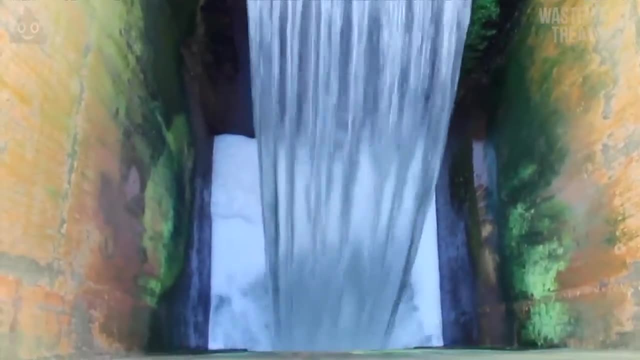 thing. Chances are you've drunk water that was waste at some point, So you might want to take some time to understand the engineering process that makes dirty water clean. So where does it start The toilet Once you're done doing your business and flush that? 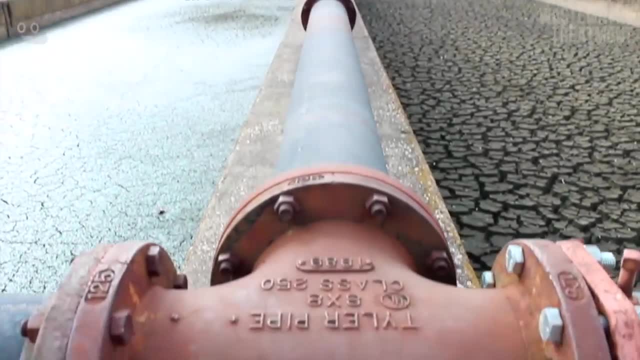 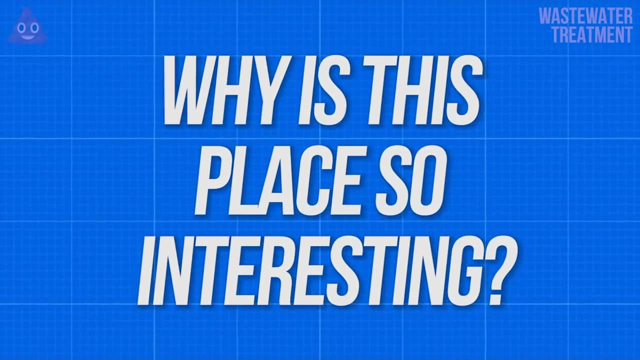 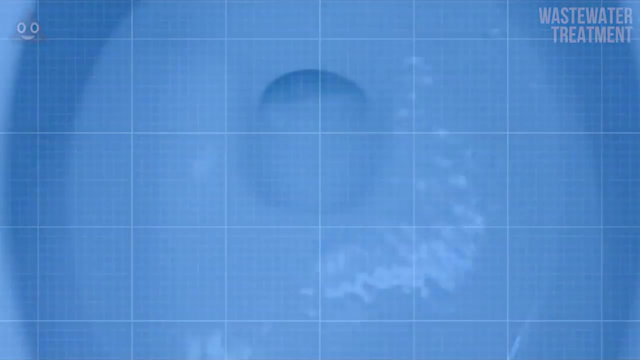 magical handle. your waste ends up at the inlet of a pretty interesting place, a wastewater treatment plant. Why is this place so interesting? Because it takes arguably one of the most disgusting substances in the world and turns it back into something that is essential to all life. Flushing your toilet at halftime may not seem like a big deal, but when you couple it. 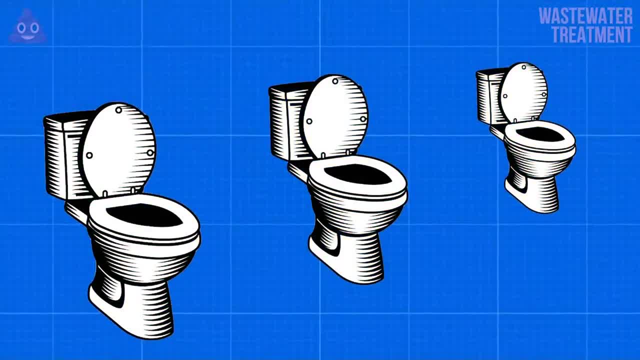 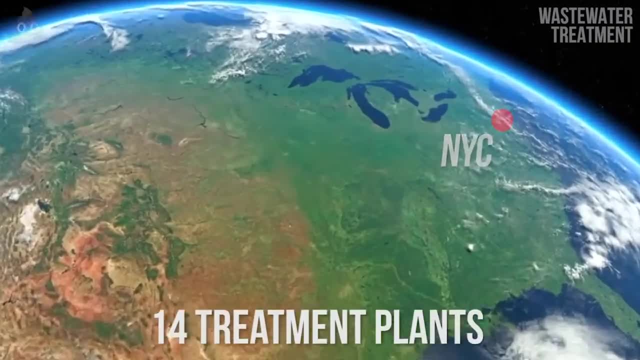 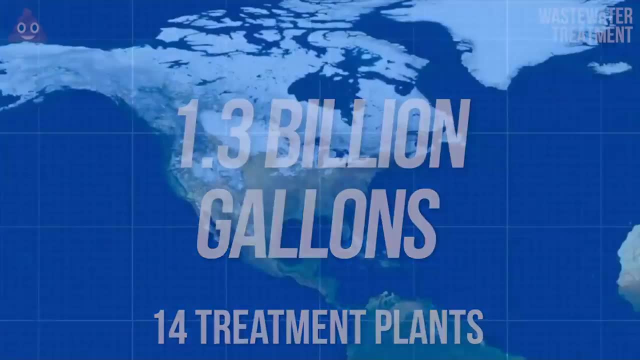 with thousands, if not millions, of others doing the same thing, it can result in some pretty high sewage flow rates. New York, for example, has an array of 14 water treatment plants that handled a combined 1.3 billion gallons of wastewater daily. That's enough wastewater to fill the Dead Sea with pure sewage in just 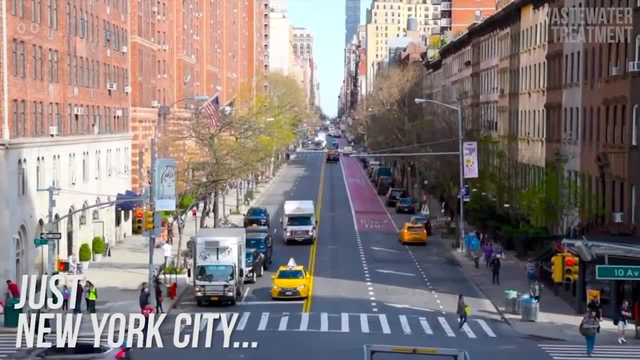 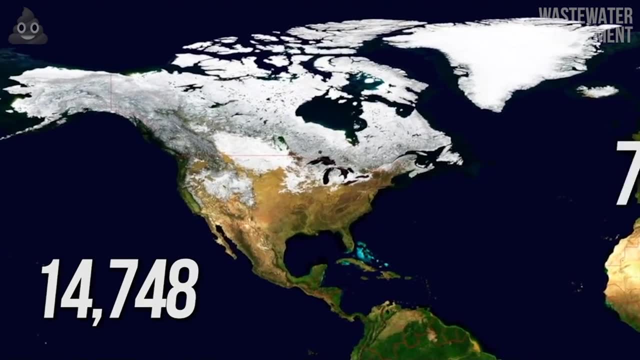 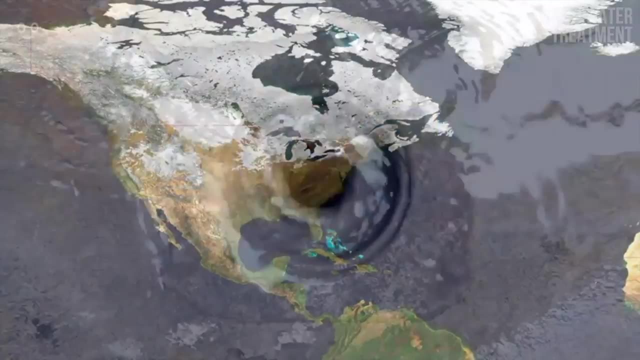 eight years. And that's just New York City. There are an estimated 14,748 treatment plants just in the US. that 76% of the US's population relies on. according to the American Society of Civil Engineers, Understanding wastewater is crucial to understanding the critical infrastructure. 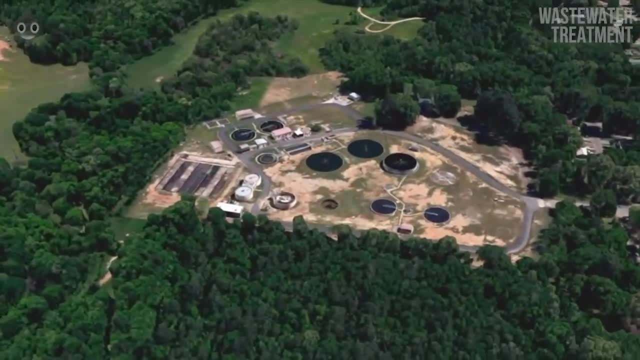 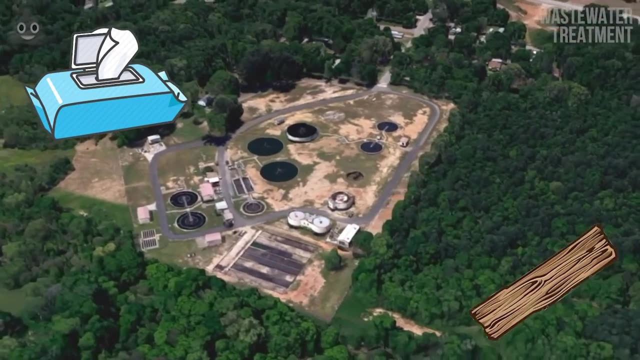 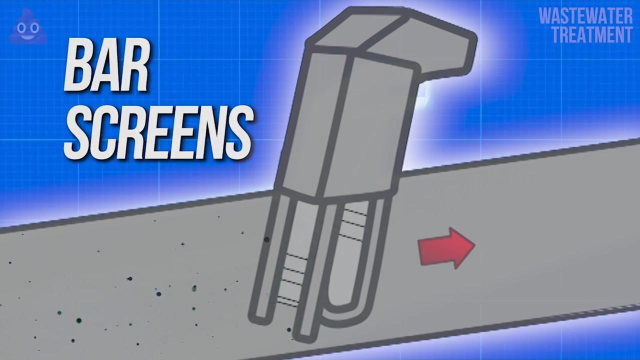 needed to support modern life. That brings us to the first step of the process that handles larger items in sewage, Things like flushable wipes, 2x4s, toys or even guns- You name it- and it's probably been caught in a bar screen. Bar screens are exactly what you would think. 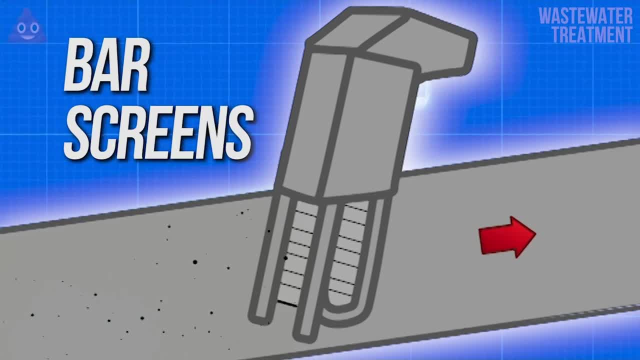 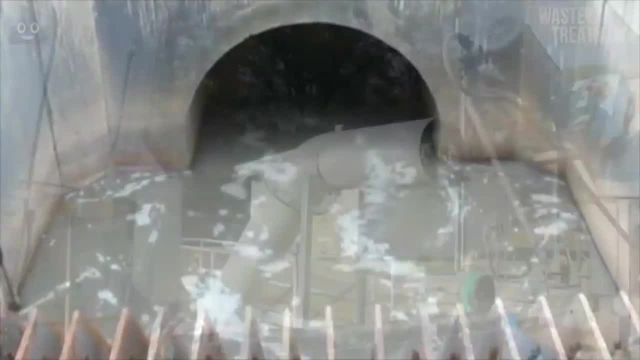 They are large vertical bars that stand at the inlet to nearly every wastewater treatment plant. designed to save lives, They stop larger items from getting to the plant and hurting machinery like pumps. The first process where bar screens are used is commonly referred to as pre-treatment. 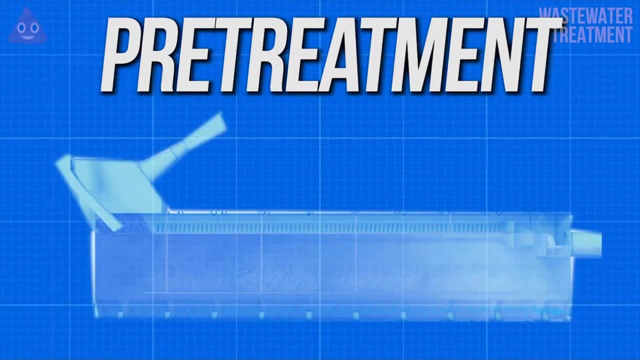 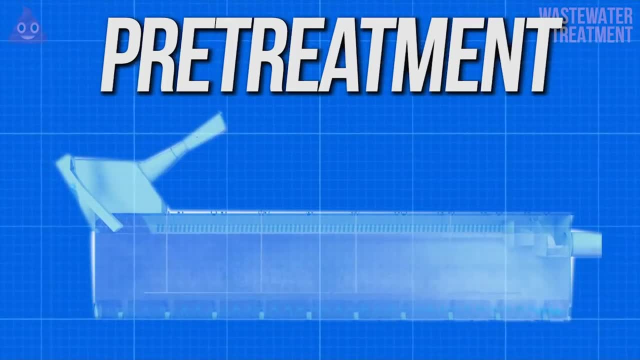 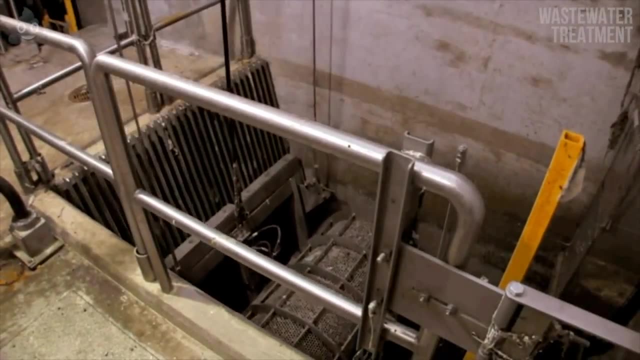 The sole intention of pre-treatment is to remove the outliers in the sewage and make the whole mixture just a little more homogenous or slightly less chunky. Bar screens are typically mechanically raked at certain intervals, depending on the flow rates of a water treatment plant. 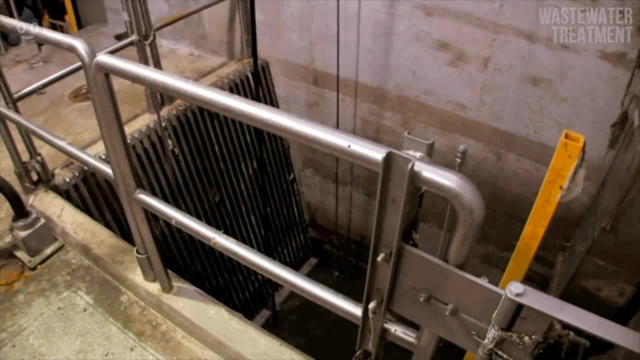 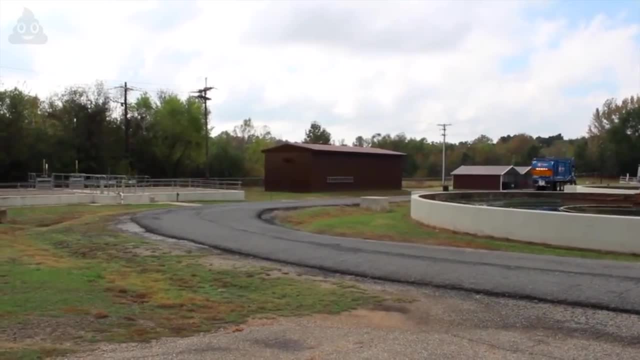 although some older plants may still have manual removal processes. Whatever is removed from the bar screens is then sent off to your average landfill or solid waste handling facility, Or, in the case of unusual items such as guns, they're sent off to the evidence locker in a 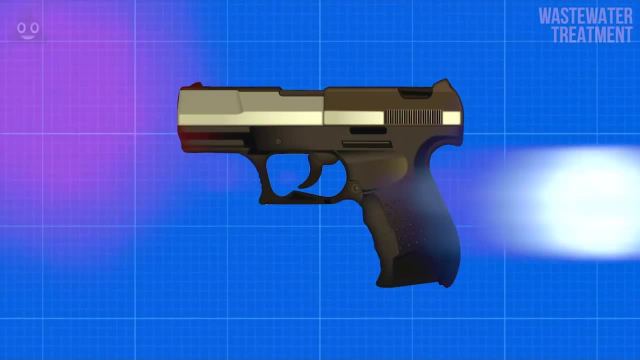 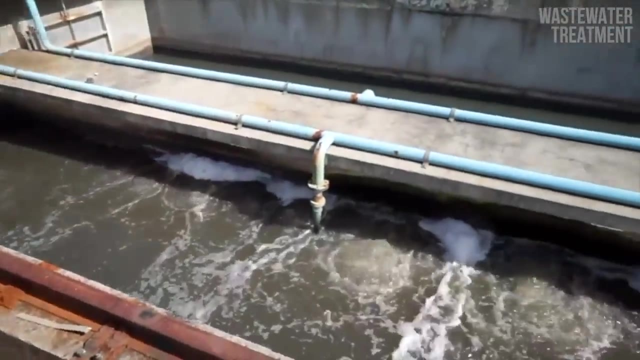 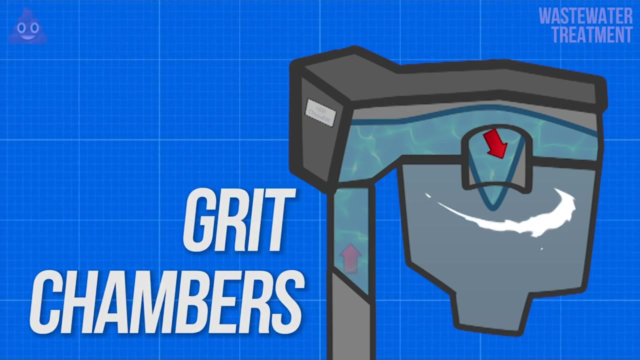 police station to be investigated. Next up is the grit chamber. No, this isn't a chamber filled with good old southern grits like your grandmother used to make. Oh no, This grit chamber is much, much worse. Grit chambers are the next step in the pre-treatment process, following bar screens, Since these. 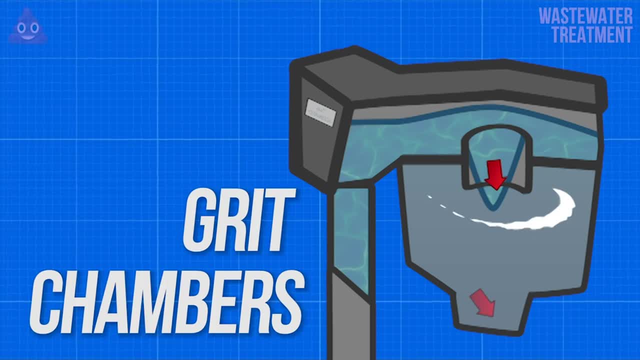 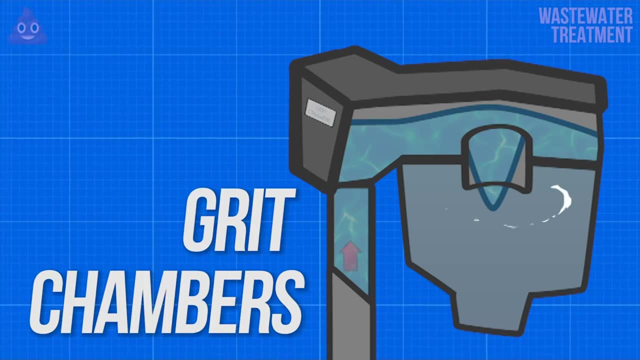 bars don't catch everything. larger particles called grit still need to be removed from the sewage as it is made even more homogenous. As the sewage flows into the grit chamber, the velocity of the rather viscous sewage is adjusted to allow for particles of sand. 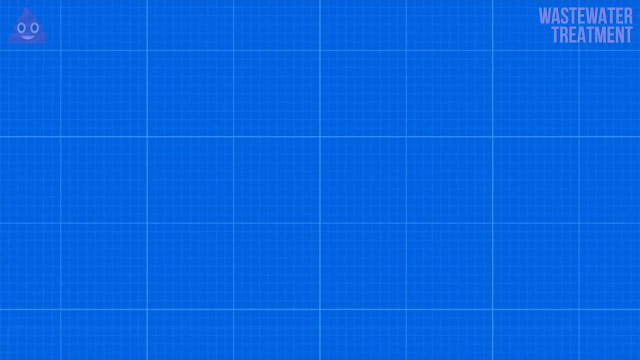 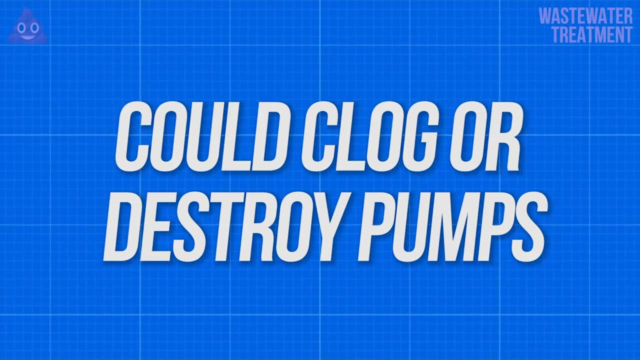 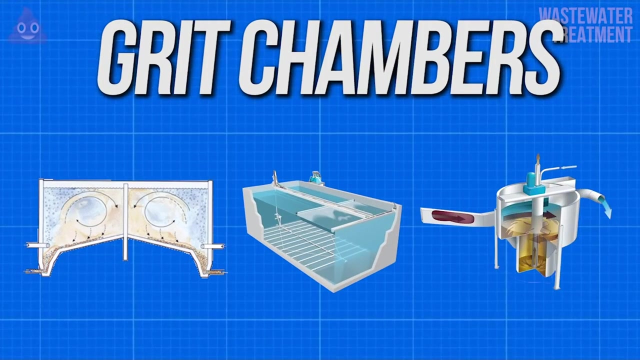 and rock to settle out. This is needed because these particles can't be removed using chemicals and they could potentially clog or destroy pumps later on. There are three types of these chambers: Horizontal grit chambers, aerated grit chambers and vortex grit chambers, which all accomplish the same task using slightly different methods. 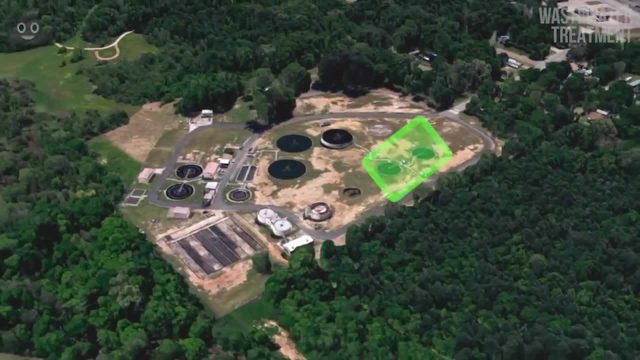 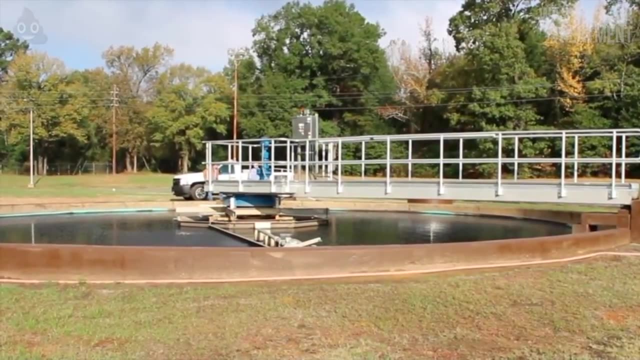 Next up are primary clarifiers. Primary treatment begins with a large basin called a primary clarifier. Primary clarifiers, and clarifiers in general, function on the principle of settling velocity. This term can be defined simply as the speed at which a particle of sand is. 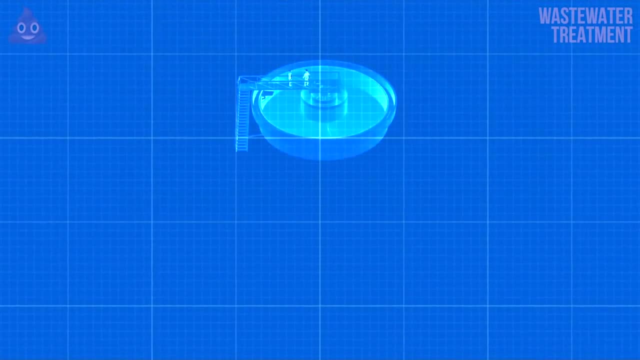 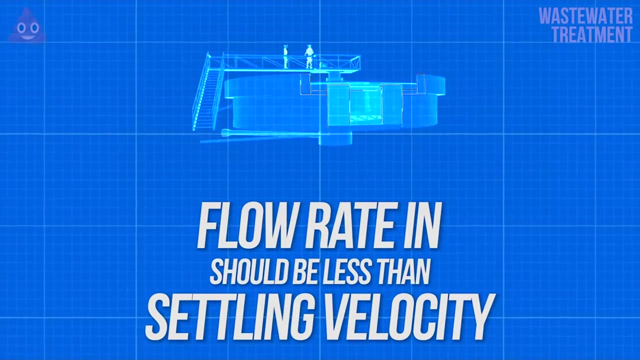 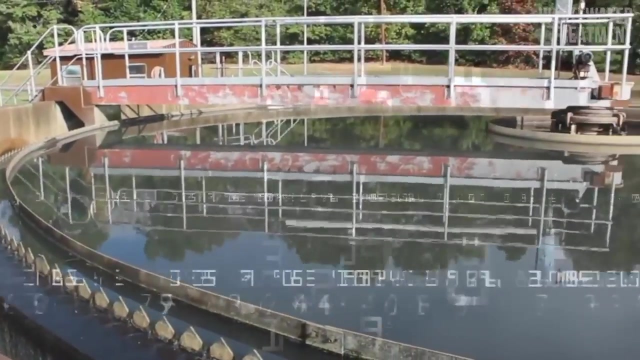 settled For wastewater being pumped into clarifiers, it's important that the flow rate of the water being pumped in doesn't exceed the settling velocity of the particles trying to be removed. In order to accomplish this, engineers will vary the size and number of primary clarifiers in accordance with a plant's permitted sewage flow rate. This 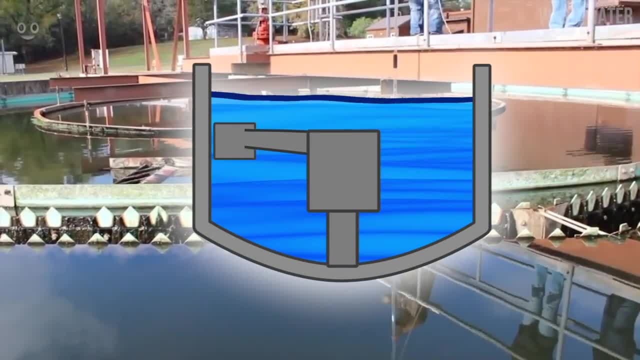 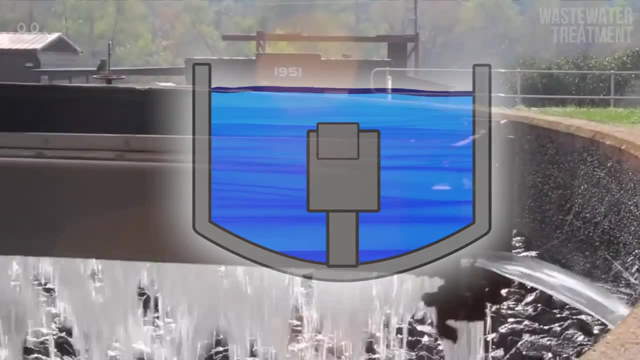 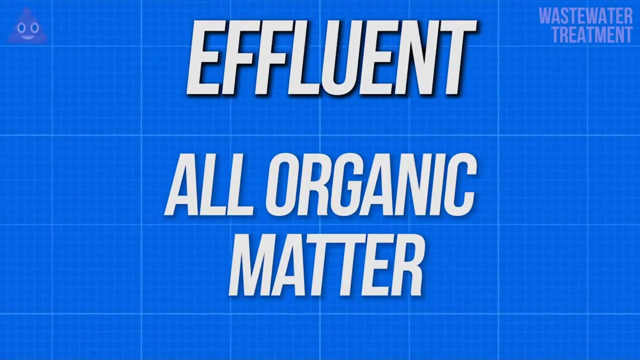 ensures that, at varying flow levels, solids can settle out of primary clarifiers to the correct quantities. At this step in the process, the slightly treated wastewater, which is referred to as effluent, is free of solids larger than 10 micrometers and should be all organic matter. 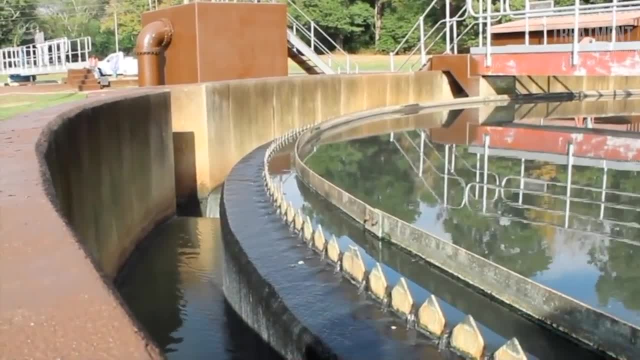 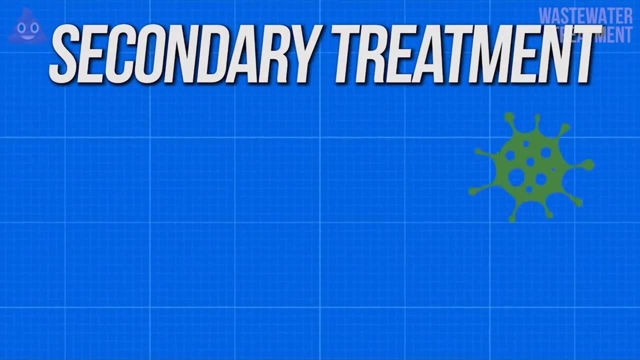 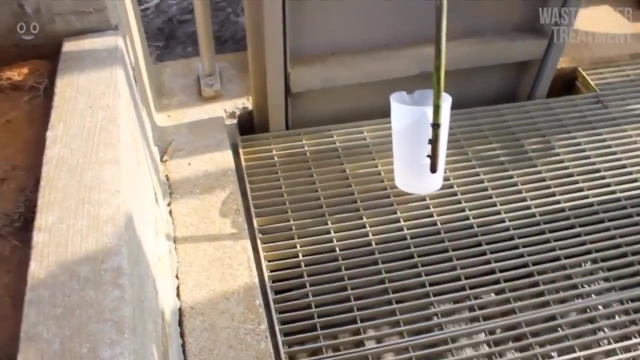 which will be treated further. The top layer of the clarified water flows over a weir wall and into the next basin. Now begins the process of secondary treatment, the sole focus of which is to significantly degrade the biological content of the sewage. In many cases, this 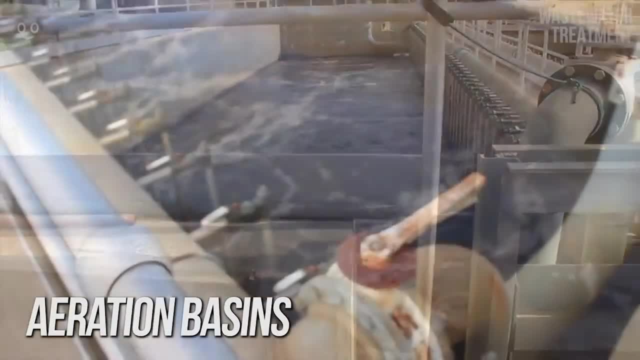 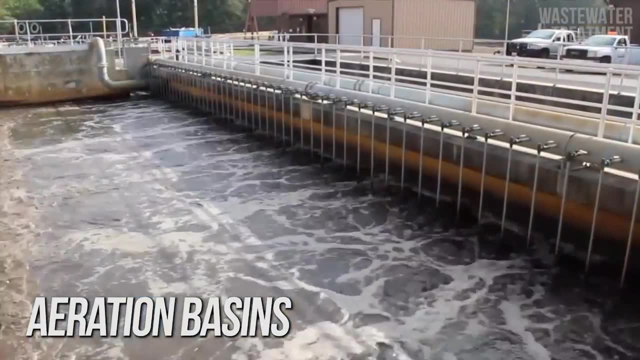 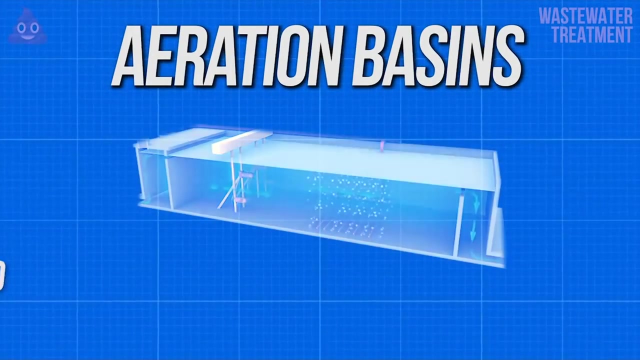 This process starts with aeration basins. Aeration basins are reminiscent of a relaxing jacuzzi tub gone awry. Effluent flows into the aeration basins, at the bottom of which are hundreds, if not thousands, of tiny air blowers that create bubbles through the water. 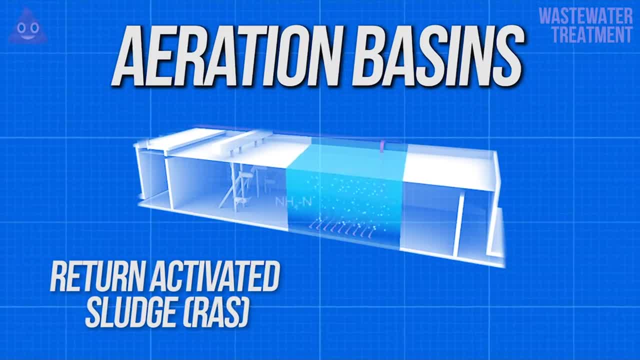 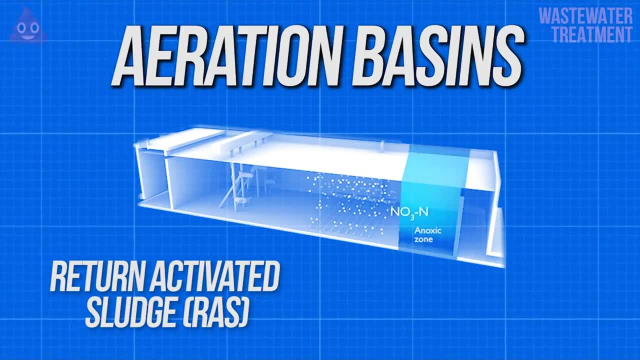 The water is pumped into this tank along with something called return-activated sludge. You can think of return-activated sludge as a bunch of happy little bacteria that get to eat their favorite foods all day long. This introduction of significant numbers of bacteria, along with the massive amounts of 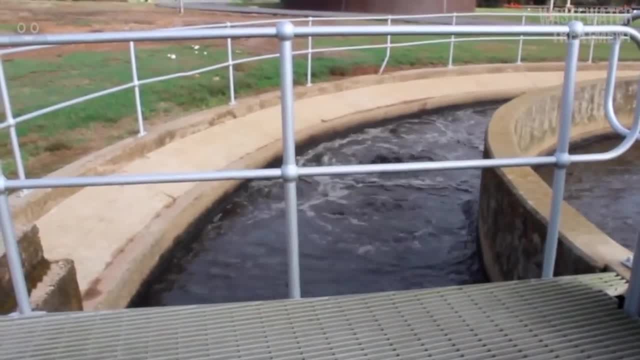 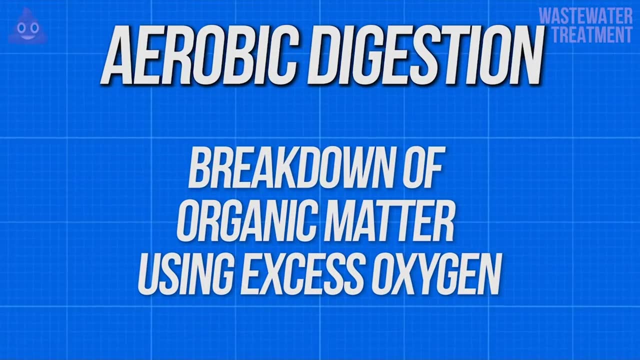 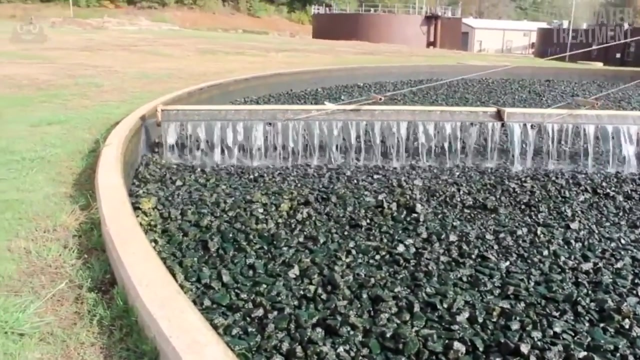 oxygen injected from the bubblers creates an environment perfect for the process of aerobic digestion. Summarized simply, it's the breakdown of organic matter along with the use of excess oxygen. Some older wastewater plants will add another step before aeration basins, referred to as 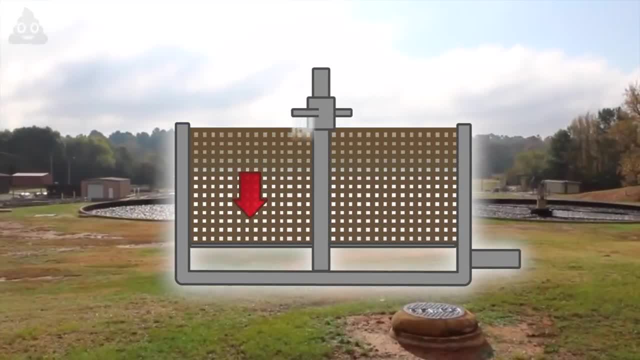 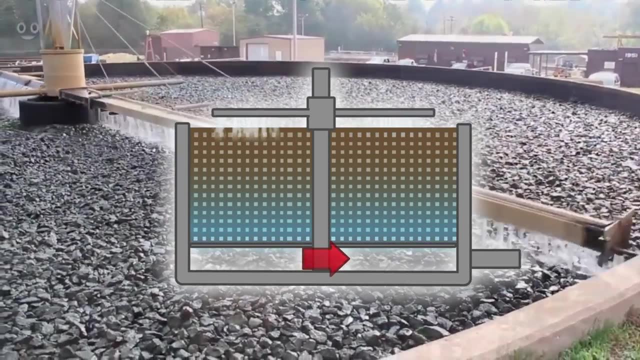 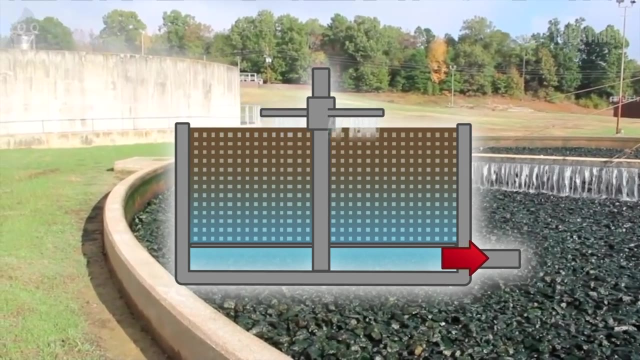 biofilters, or trickling filters, Found in many older plants. these filters essentially trickle the effluent over a medium like stone or plastic and allow for a film of bacteria to chow down on any organic matter in the water. This step is largely not used in newer plants due to more efficient and modern processes. 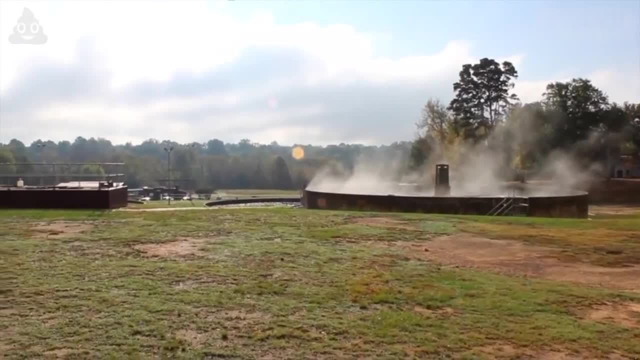 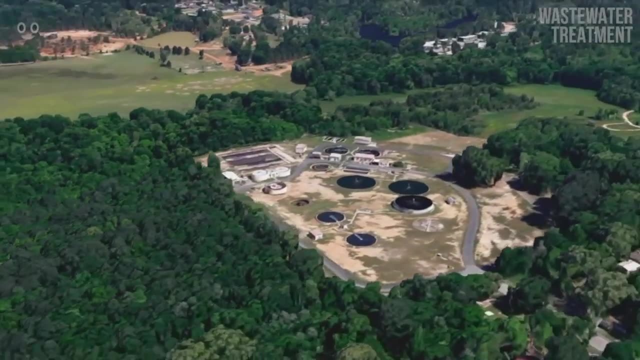 but for plants with the basins already installed, many still use them because they only benefit the treatment process. in most cases, Following the aeration basin, the effluent, along with much of the sludge, is pumped into a secondary filter or clarifier, where some of the sludge is removed and pumped back. 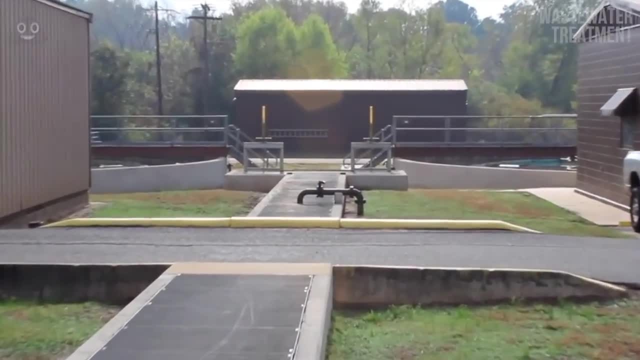 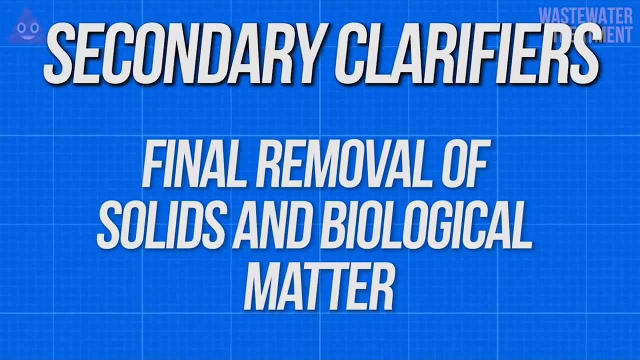 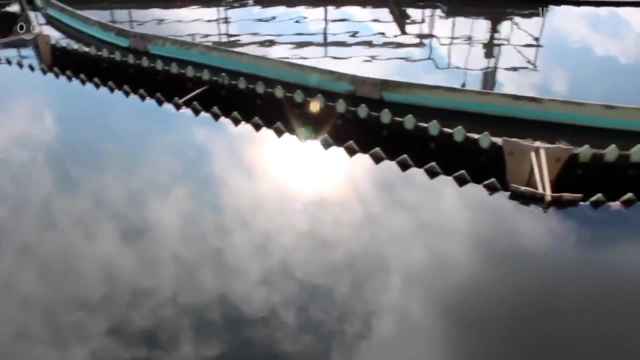 into the aeration basins as the return activated sludge. Further settling of larger particles is also accomplished in these basins, as it is the final step of the process to removing solids and larger biological matter. Water flows out of secondary clarifiers over a nearly identical weir wall to the primary. 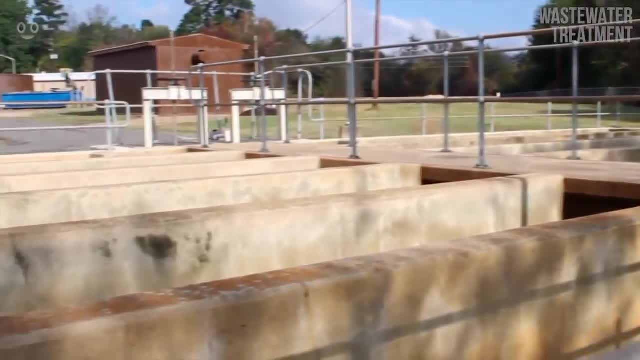 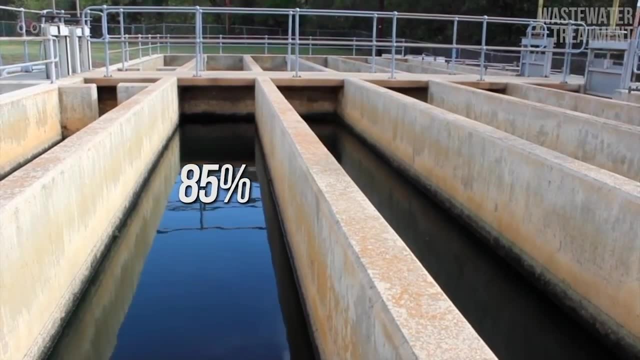 clarifiers and moves on to the disinfection process. At this point, 85% of the water is removed, 85% of all organic matter is removed from the water and the effluent is safe to drink in most cases, although you wouldn't want to. 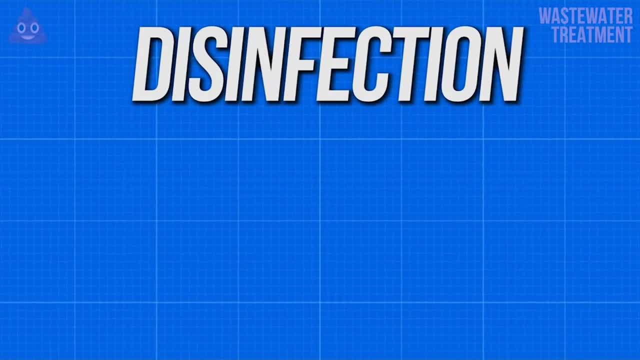 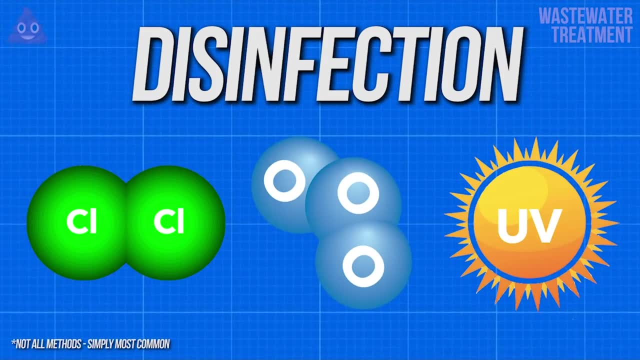 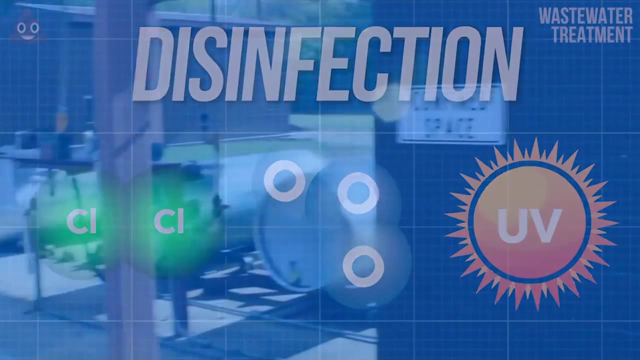 Disinfection is the final step in the process and is usually accomplished in one of three ways, either through chlorine, ozone or ultraviolet disinfection. Each process has its benefits and drawbacks, with each being used commonly throughout the wastewater treatment process across the world. 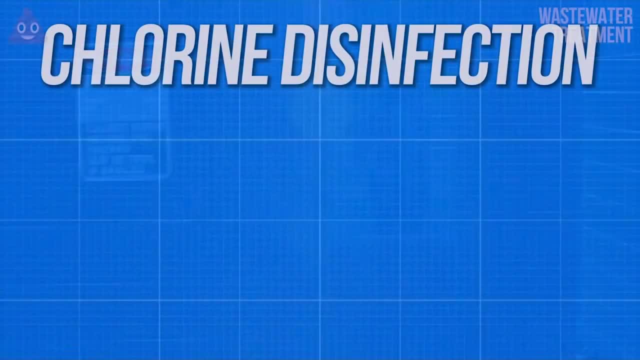 Chlorine disinfects the water through chemicals. Chlorine is a chemical that is used to clean the water. Chlorine is a chemical that is used to clean the water. Chlorine is a chemical that is used to clean the water. Chlorine, which you can think of as concentrated bleach, is added to the effluent here to kill. 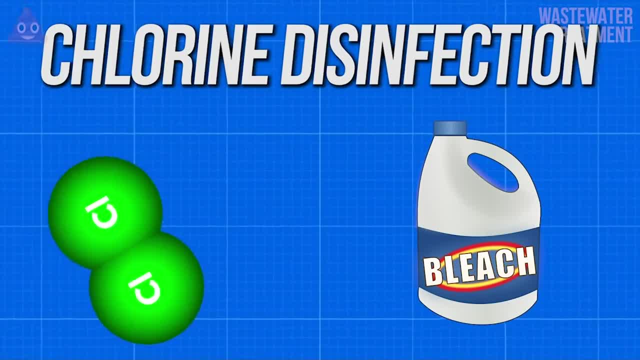 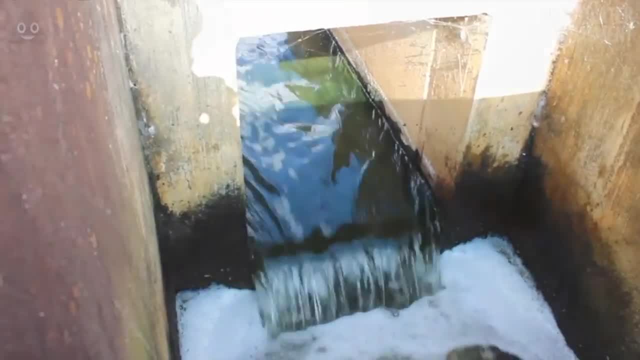 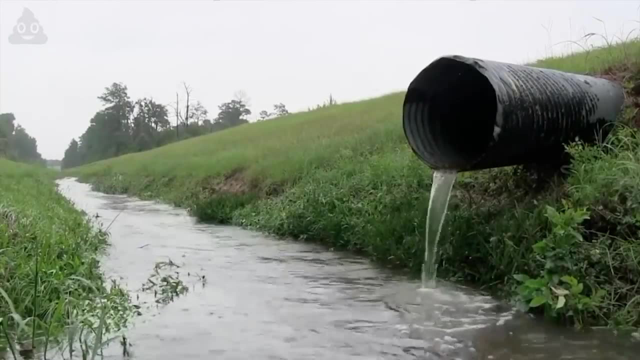 off any remaining bacteria and organisms still living in the water. When chlorine is added to kill off the bacteria, it then has to be removed before it can be discharged, as to not kill off anything in the discharge location like a pond. After this, the water is safe enough to discharge. 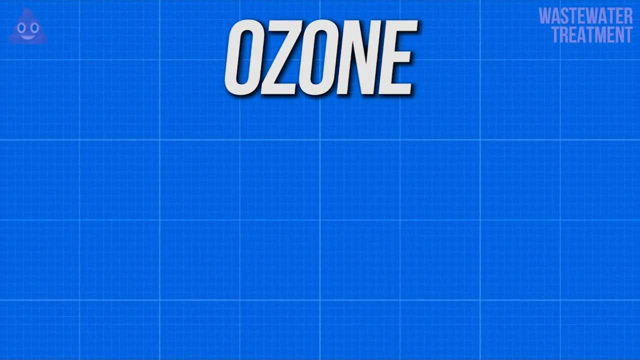 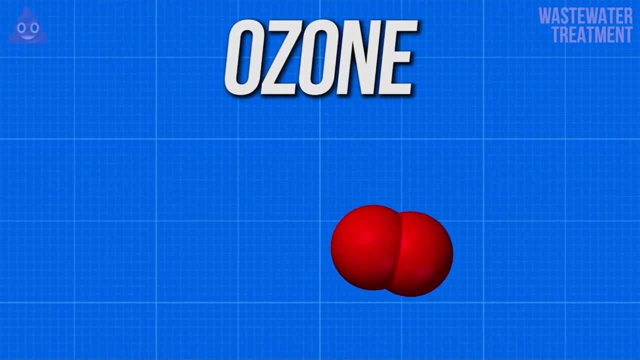 Ozone disinfection is another method of chemical disinfection that involves pumping and emptying an electrical current through the water. that causes oxygen molecules- or O2, to disassociate and combine with a free oxygen molecule, forming O3, known as ozone. 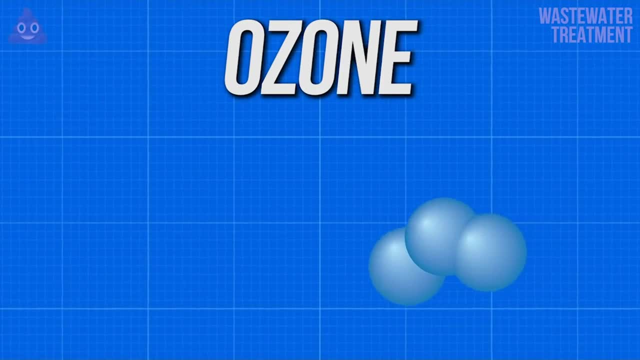 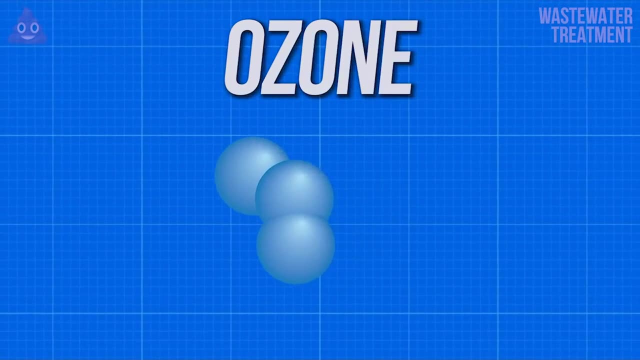 Ozone is an incredibly strong oxidant and causes microbes' cell walls to leak, rapid cell decomposition and overall damage to cells. In other words, it kills off the bacteria. The last common disinfection method uses ultraviolet light to scramble bacteria's DNA. 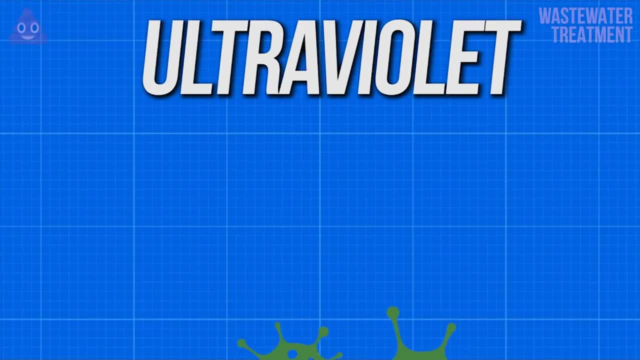 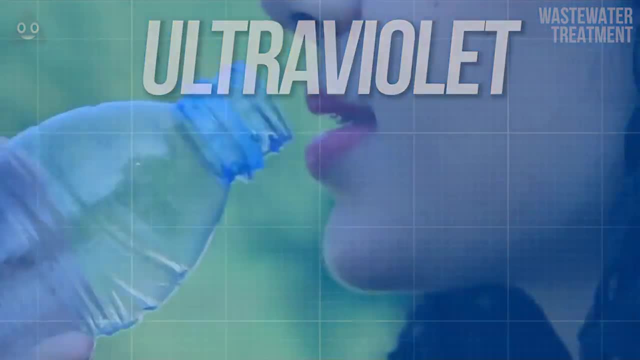 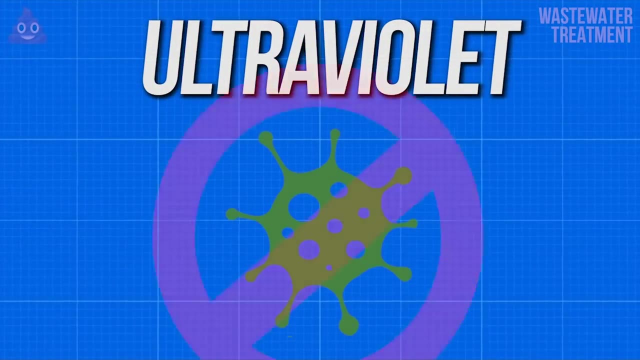 So they can never reproduce. In UV disinfection, the bacteria in the water aren't killed. rather, they are sterilized, rendering them harmless. If you were to ingest water with living microbes immediately following UV treatment, any harmful bacteria would be unable to multiply or render your body damage. 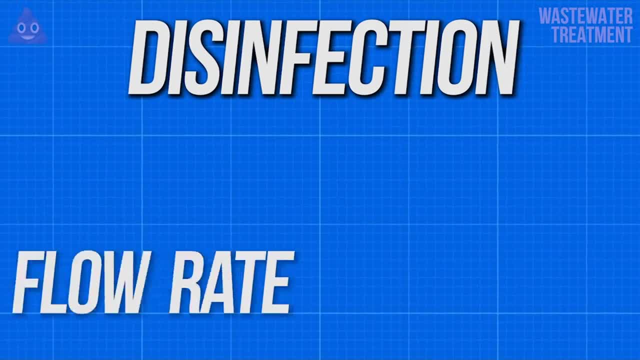 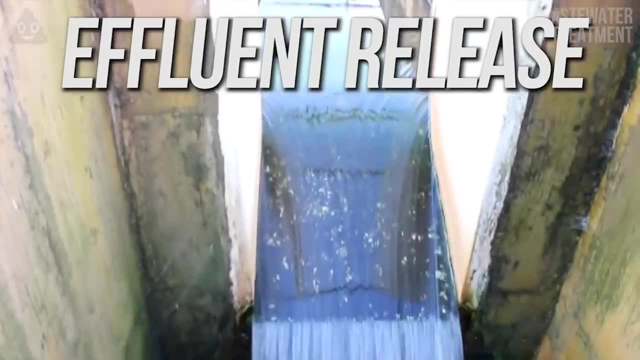 Engineers choose between these methods based on a variety of factors, such as flow rate, cost and location of discharge. So what are the most common types of Ozone disinfection methods? First, the most common type is effluent release. Effluent release is an effective way to release a new form of water: water that is not to